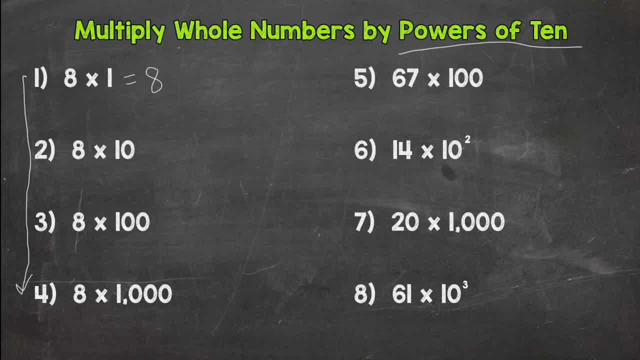 is 8. again, 1 is not a power of 10. the powers of 10 are 10, 100, 1000, 10, 000, 100, 000, a million and so on. so let's go to number two: 8 times 10. think to yourself what's 8 times 10? 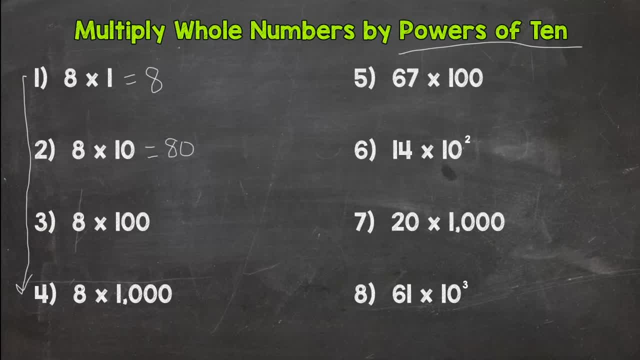 hopefully you're thinking 80. right, let's do 8 times 100. 8 times 100 is 800, and then let's finish off with 8 times a thousand and that's going to give us 8,000. simple enough, right? I'm going to line all these answers up over here to the right, and I want you. 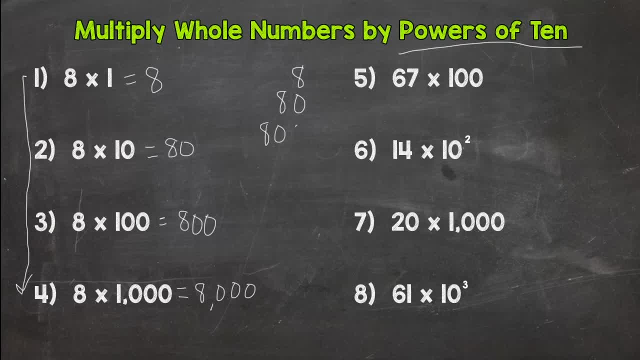 to take a look at where the 8 is placed as we go down through these answers. so 8 times 1, we have 8. then we have 8 times 10. what place did the 8 move to? it moved over to the tens place right. and what did we use to bump the 8 over to the tens place? we used a 0. 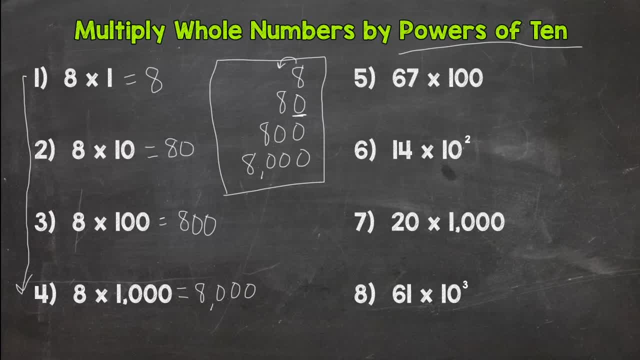 how about 800? we move the 8 to the left again, 8 times 100, and the 8 is in the hundreds place. what did we use to bump the 8 over to the hundreds place place Two zeros. And then how about eight times a thousand? We get eight thousand, And 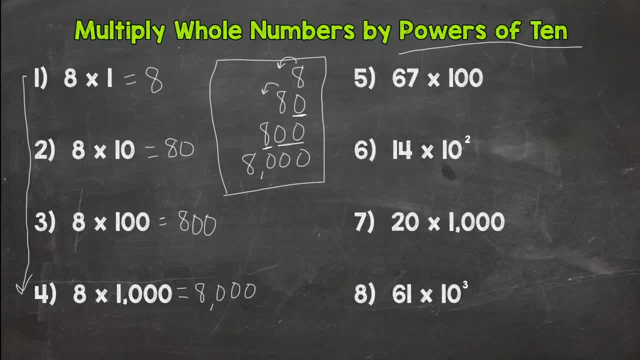 the eight is in the thousands place. What did we use to bump the eight over to the correct place value? We used three zeros. Now notice: three zeros in a thousand. guess how many zeros were in my answer. Two zeros in a hundred. guess how many zeros I used to bump everything. 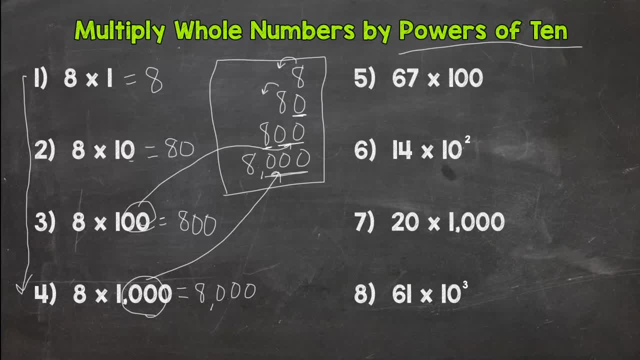 to the correct place value Two. One zero in ten. How many zeros did I put on the end of eight to bump it to the correct place value, One? So whenever you're multiplying by a power of ten, all you're doing is moving your digits to the left in the place value chart to increase. 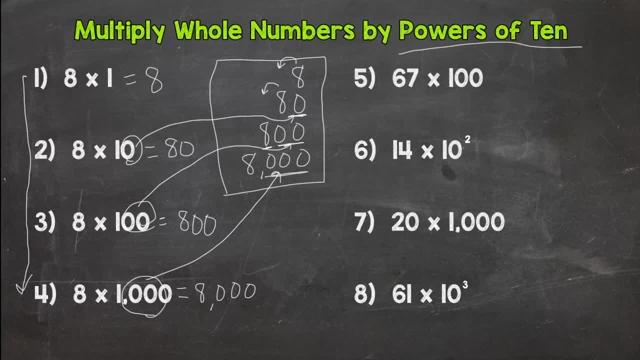 the value. And we do that by putting zeros on the end to push everything to the right spot. So let's look at number five. here We have sixty-seven times a hundred. So all this is saying is we are pushing sixty-seven. 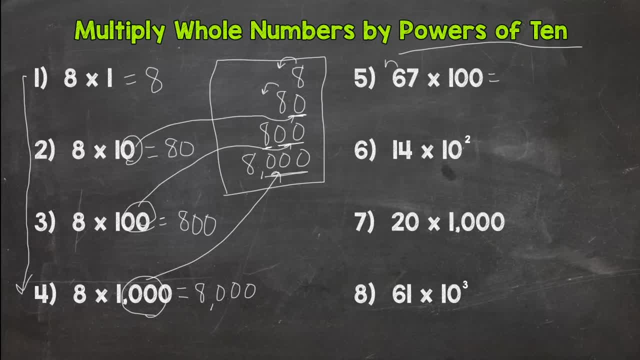 the six is going to go two spots to the left and the seven is going to go two spots to the left, And we put two zeros on the end of sixty-seven in order to do that. One hundred has two zeros, so we put two zeros on this end of sixty-seven to push it to the right. 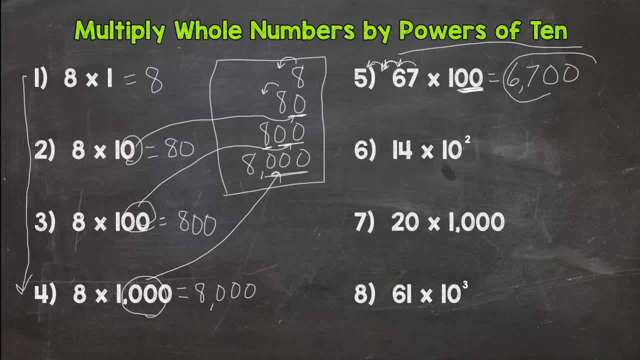 So we put two zeros on the end of sixty-seven to push it to the right spot and we get six thousand seven hundred. Now, an easy way of explaining this is: I just add two zeros to the end of sixty-seven. Well, that's true, but it really doesn't show that we understand. 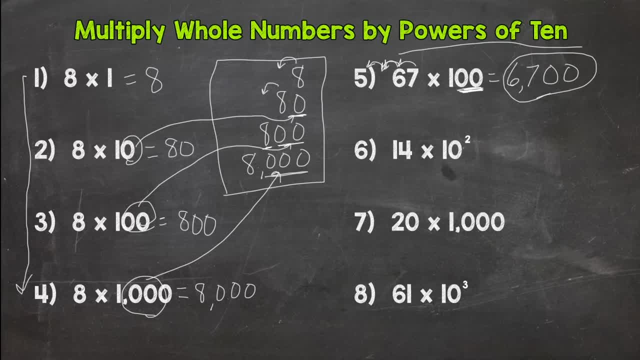 what we are doing. If you want to think of it like that, that's fine, But make sure you understand that we put the two zeros on the end of sixty-seven in order to push everything to the correct place value, so we get the correct answer. okay, Think back to a simpler problem. I'll 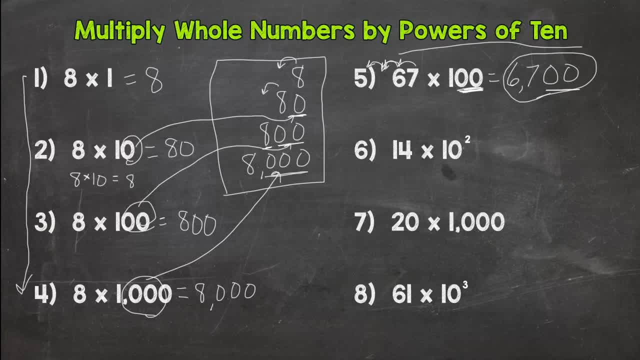 come back to this: 8 times 10 is 80, right, We all know. 10 plus 10 plus 10, 8 times equals 80, or 8 times 10 is 80. We used 1, 0 to push that 8 to the correct spot, to the correct place. value okay. 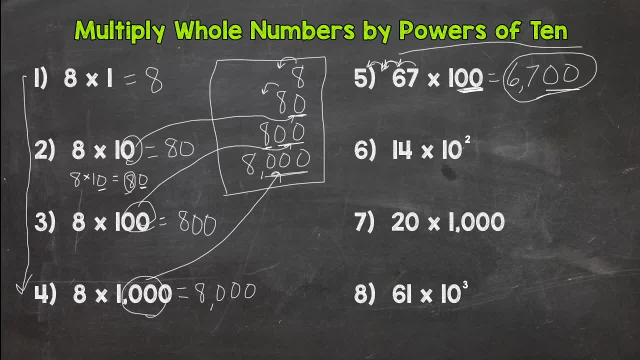 Now number 6, we have 14 times 10 squared, or 14 times 10 to the second power. Well, we have to think about what 10 to the second power is. 10 to the second power means 10 times 10, expand it out. 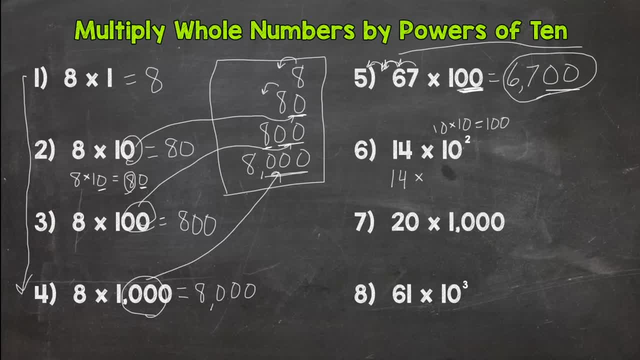 right, And 10 times 10 is 100.. Exponent of 2, expand 10 out twice two 0s in our 100.. So all this means is 14 times 100.. So how many 0s? 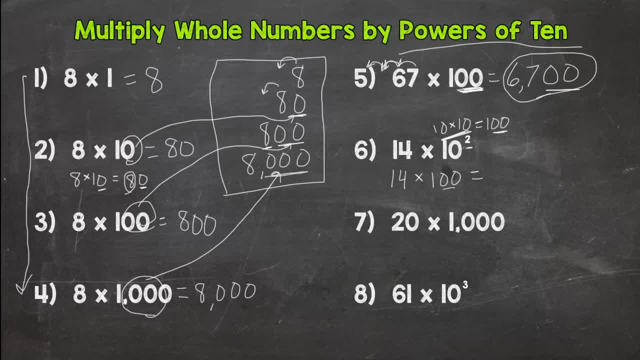 Do we put on the end of 14 to push it to the correct place value? Well, 2.. So all we need to do is put two 0s on the end of 14, and it will give us the correct answer. Our answer is 1,400.. 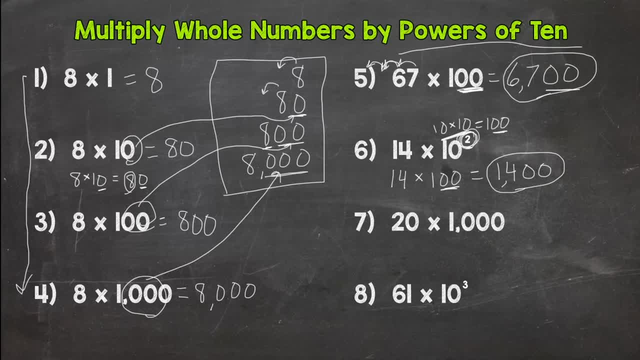 Now, when you have these exponents, look, we have a 2 here. That means two 0s on the end. okay, That exponent just tells you how many 0s you need to put on the end to push everything to the correct place value. So number 7 is a very, very important one, because we have a 20 here. 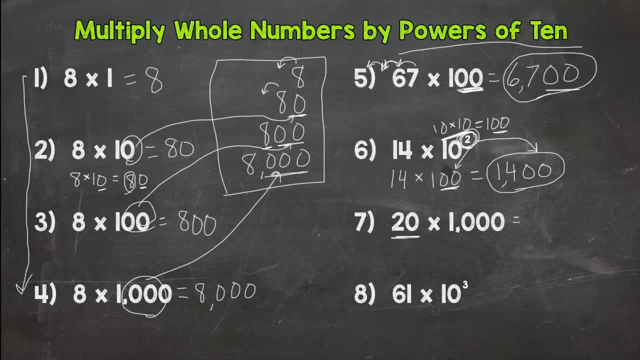 It already has a 0 on the end, but we need to push that two 3 spaces to the left and we need to push that 0, 3 spaces to the left, So we need to put an additional three 0s on the end of 20 to get everything to the right place value. 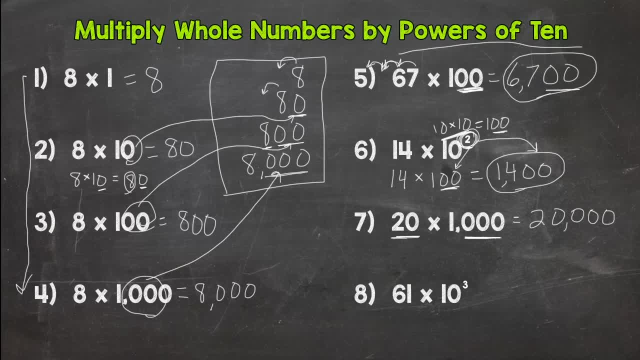 So we need 1,, 2,, 3.. We get 20,000,. okay, Don't do this. Don't just put three total 0s. That would give us 2,000.. Is that the same as 20,000? No, And you got to think what makes sense. 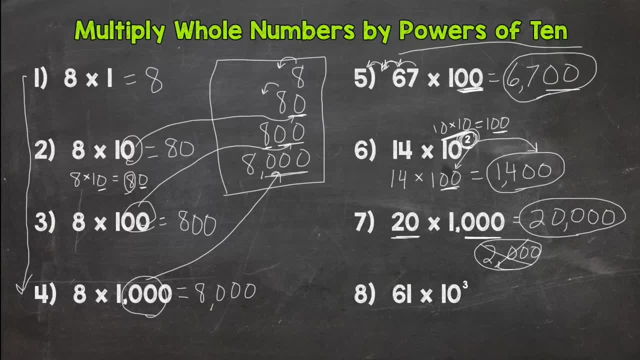 Well, 20 times 1,000 wouldn't give you 2,000.. 2 times 1,000 equals 1,000.. 20 times 1,000 equals 20,000.. Makes sense and it is our correct answer. So let's go to number 8.. 61 times 10 to the third. 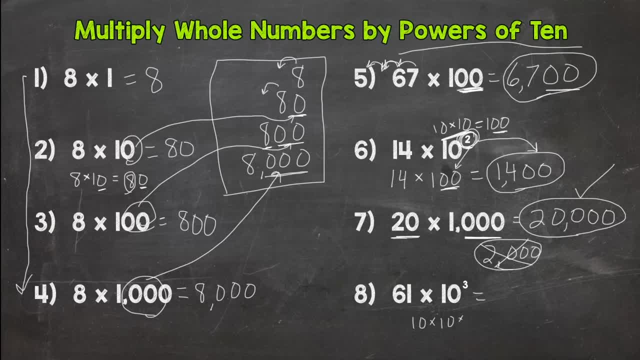 power, which 10 to the third power means 10 times 10 times 10,, which is 1,000. So we have 61 times 1,000.. So we have our 61, and then we need our three 0s on the end to push it all to the correct. 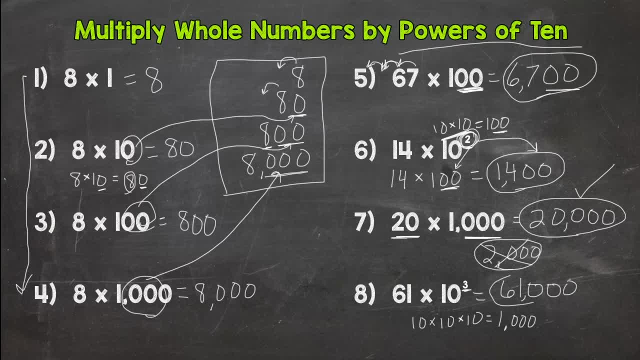 place values and we have 61,000. So that's multiplying whole numbers by powers of 10.. You use 0s to push everything to the correct spot and you look back at your original problem. You check what the exponent is, or. 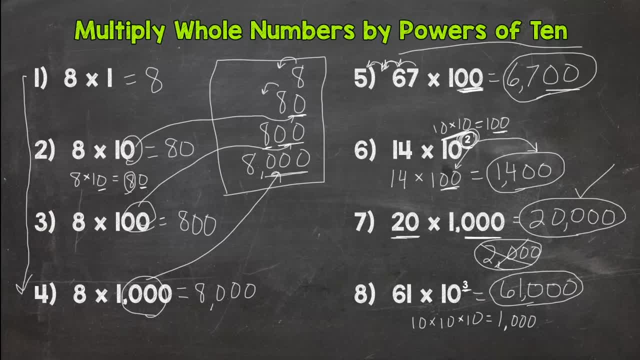 how many 0s are in your power of 10, and that will match how many 0s you need to put on to your answer. Okay, So that's multiplying whole numbers by powers of 10.. It's time for you to try some on your own.